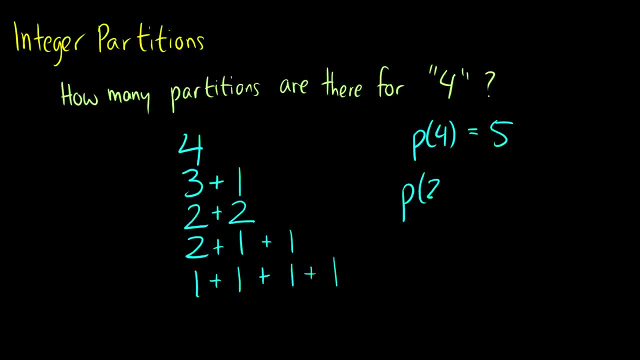 exhaustive if I say what is p of 26, because there's a ton of options. So instead we're going to work with generating functions. Now, how do we figure out what the generating function for this is? Well, we take a look at how many ones there are, how many twos, there are threes and so on. So if we take 0, 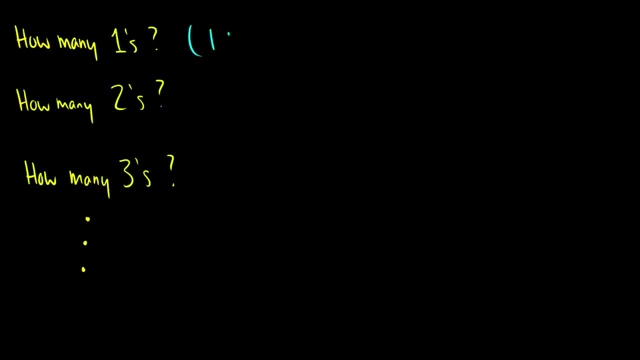 ones, we just get x to the 0, which is 1.. If we take 1 1, we get x to the 1.. If we take 2 ones, we get x squared, and, of course, this is just your 1 over 1 minus. 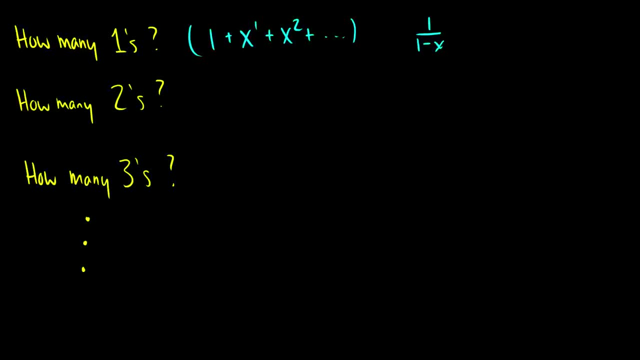 x Generating function. How many twos? Well, if we select 0 twos, we get 1.. If we select 1- 2, we get x squared, because we want essentially these coefficients or these exponents to add up to whatever number we're looking at. So if we select, 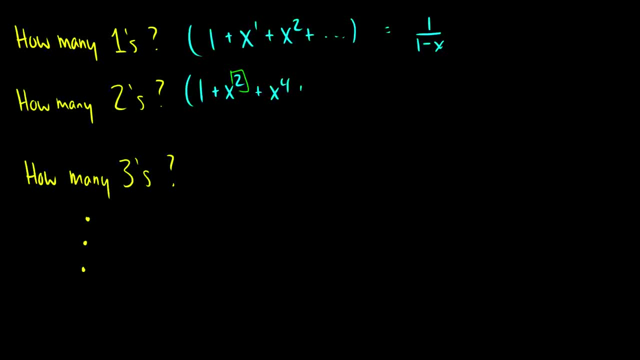 2, twos, we get x to the 4, plus dot, dot, dot. So this is just the same as 1 over 1 minus x squared. How many threes? Well, same logic: we pick 1, 3, we get x, cubed. we pick 2 threes, we get x, 6, so on. So this: 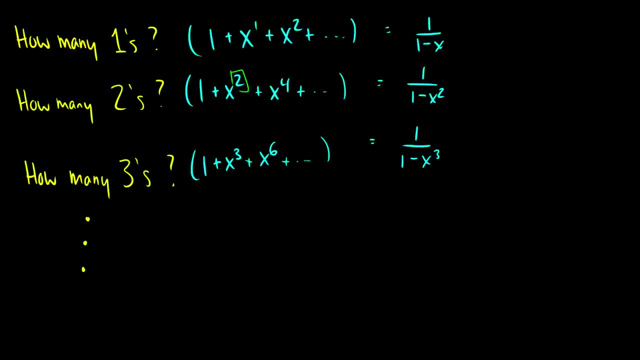 is just 1 over 1 minus x cubed, and clearly this is just going to go on for forever. So when we say how many n's are there, well that's just going to be 1 over 1 minus x to the n. So that's how we take a look at partitions. So in general, if we 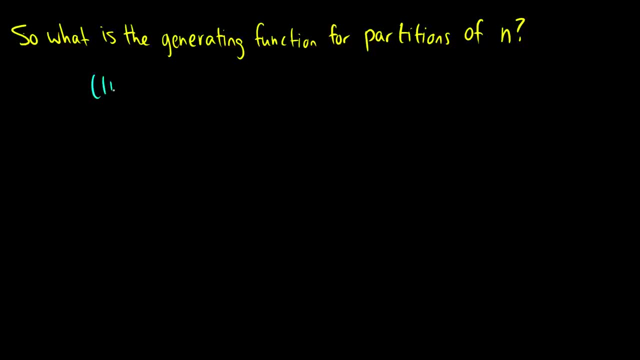 look at the number of partitions for n. this is going to be the generating function for the number of ones times the generating function for the number of twos, then the threes, then the fours, all the way up until however high we want to. 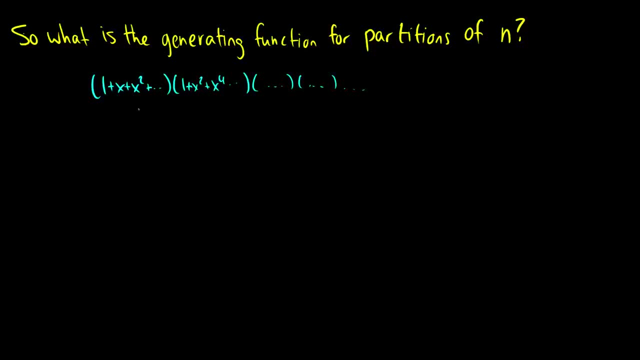 go. So what this really is is 1 over 1 minus x, times 1 over 1 minus x squared, times 1 over 1 minus x cubed, and that goes on for 1 over 1 minus x to the n, and then it keeps going. So we have a nicer. 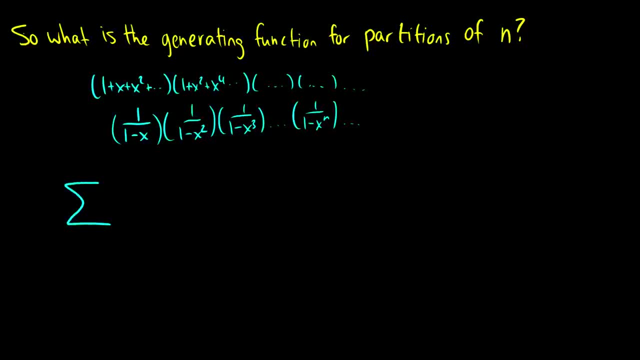 notation for this and if you remember the sigma notation, we can say that i is greater than 0 of x to the i times a, i, which is just a formal power series. Well, we have a new symbol for multiplication instead of addition, because sigma is the. 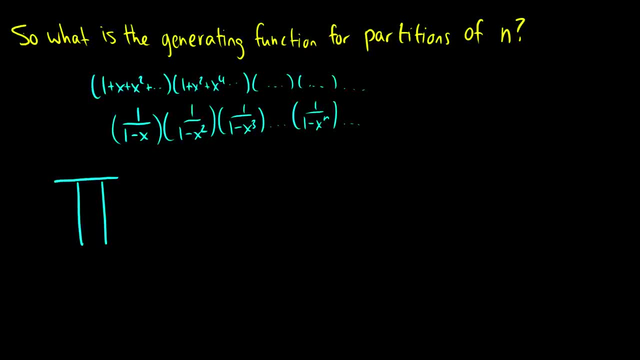 sum pi is the product. So we say i is equal to 0 to infinity. in fact I can just say i is greater than or equal to 0.. In fact it really should be: i is equal or greater to 1 in this. 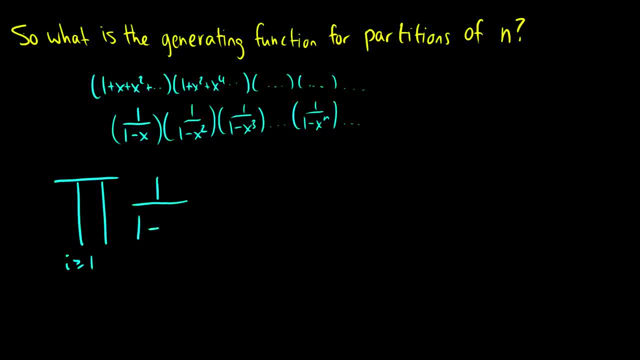 case of 1 over 1 minus x to the i. So that's 1 over 1 minus x to the, 1 times 1 over 1 minus x, squared times 1 over 1 minus x cubed, so on. So 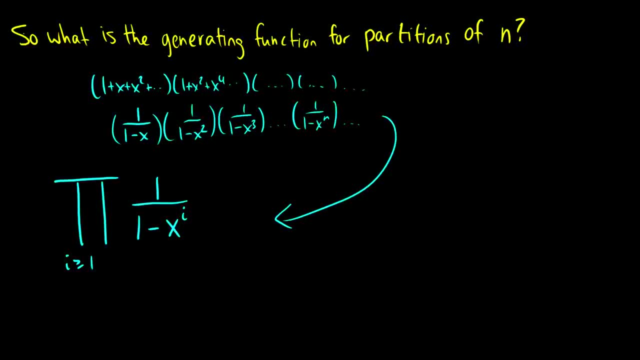 that product is equal to this notation. It's just a nicer way of writing things out. So that's the generating function for partitions of n, and of course, the value you're looking at is going to be the nth coefficient. So we know that the 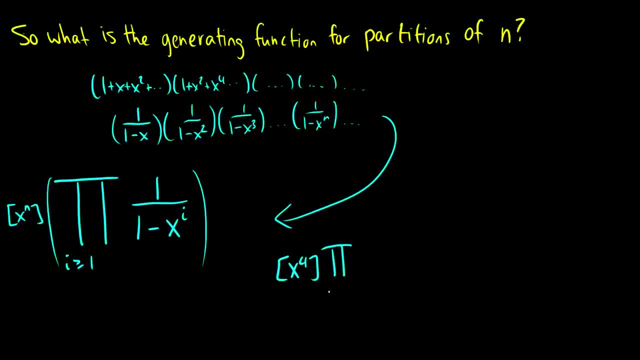 fourth coefficient of the generating function, for i equals one to It would be four of 1 over 1 minus x to the i is just going to be 5.. We wouldn't expect you to actually find this, because this is not an easy thing to compute, So it's more. 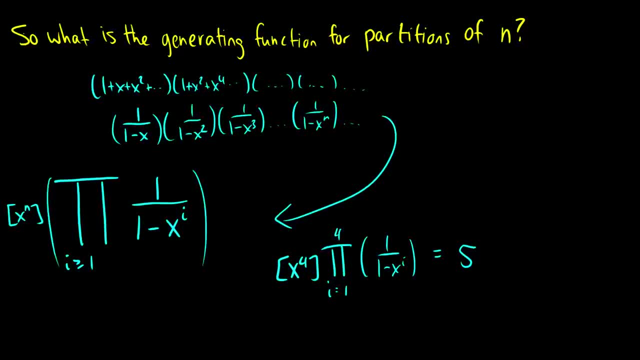 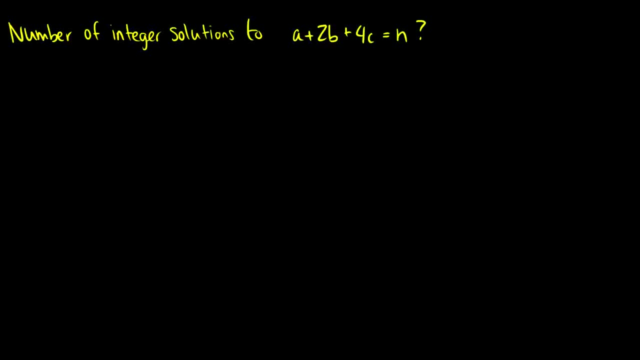 like saying: what is the generating function? Don't worry about the coefficient, because a computer can find it for you. So now that we've done that, let's take a look at another cool thing we can do with it. Before we've had x1 plus x2 plus x3 is equal to n, and we know that's just 3 plus n minus 1. choose n. 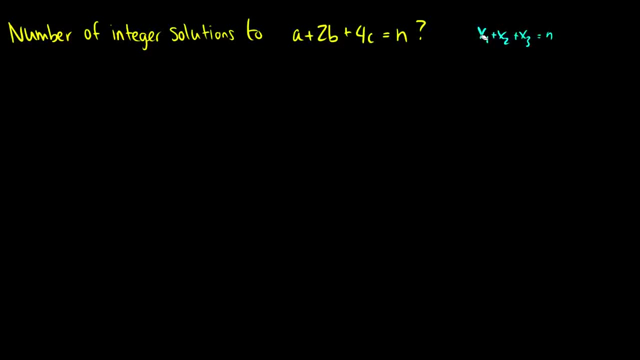 But what happens when we put coefficients in front of those? So instead I say: oh, what about ax1 plus bx2 plus cx3 is equal to n. Well, that gets trickier, so we just use generating functions. Okay, so in this case a, b and c- all are greater or equal to 0, so I should probably write that down. 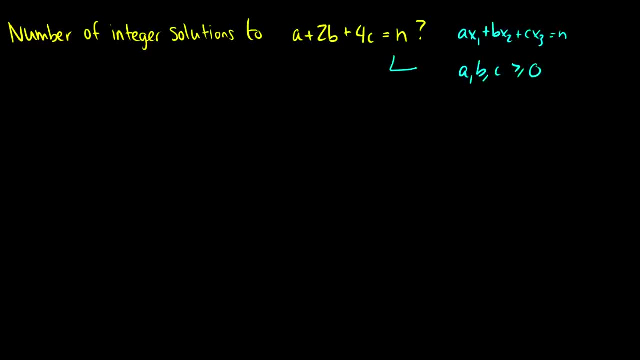 a, b, c are going to be greater or equal to 0 for this example, And what we want is: we want the nth coefficient of some generating function, And we don't really know what it is yet, so let's figure it out. 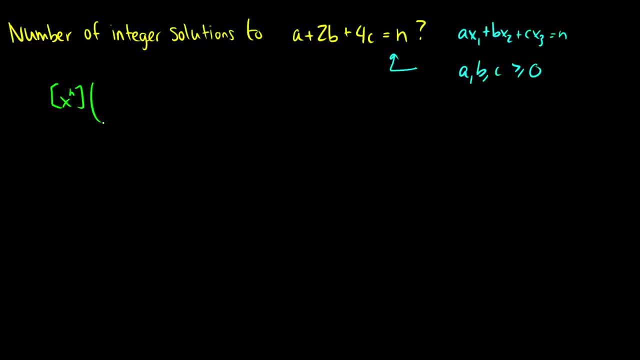 Well, a, let's pick. Let's pick a number for a. so 1 plus x, plus x2 plus x3, it can really be anything, because it's just a. But what about 2 times b? Well, b is just like a, except whatever you pick is multiplied by 2, which means if we pick x0, it's just going to be x0.. 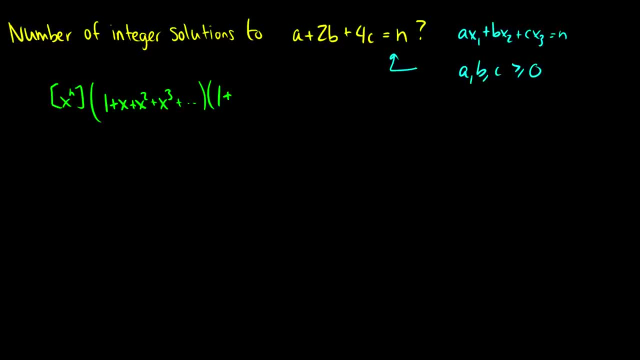 But if we pick x1, it can't be x2.. It has to be x1,, it has to be x2, so x squared, Then we have x to the 4 plus x to the 6, so on and so forth. 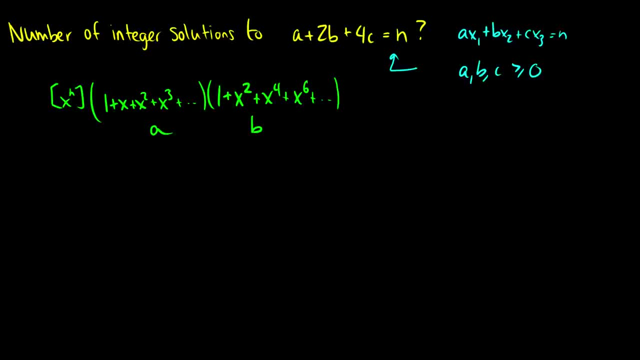 So this is our a, this is our b. And now, what do you think we do for 4c? Well, for 4c again, if we pick x0, we just get x0 back when we multiply it by 4.. 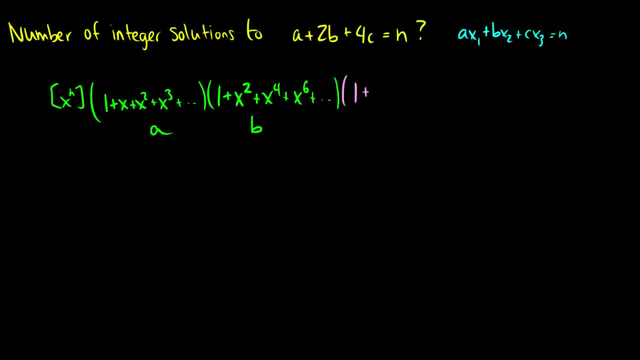 But if we pick one object, we're actually picking 4.. So we get x to the 4.. If we pick two objects, because we're multiplying by 4, we get 8, so we get x to the 8.. 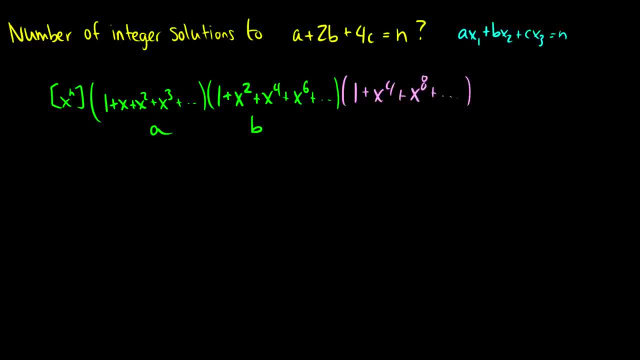 And that just goes on forever. So we want the nth coefficient of a times b, times c, And of course we can shorten this to 1 over 1 minus x. So this is x to the n of 1 over 1 minus x. 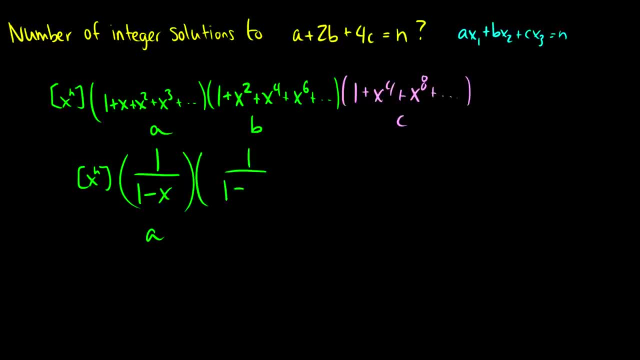 Of course, this is the a's, 1 over 1 minus x squared for the b's, And we can shorten this to 1 over 1 minus x squared for the b's, And 1 over 1 minus x to the 4 for the c's. 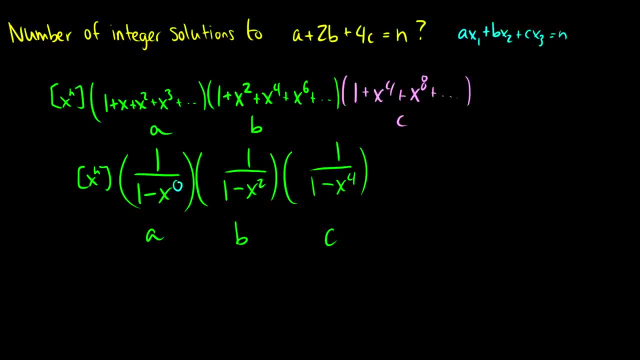 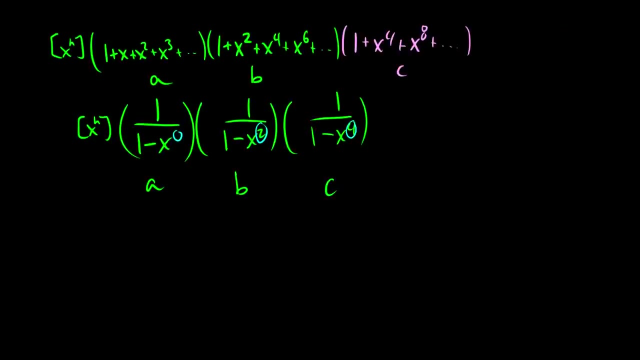 Clearly you can see here that the coefficients match up with the coefficient of the a's, the b's and the c's. So if we have say: what if I just said, let's pick a nice new example here, I want 18a. 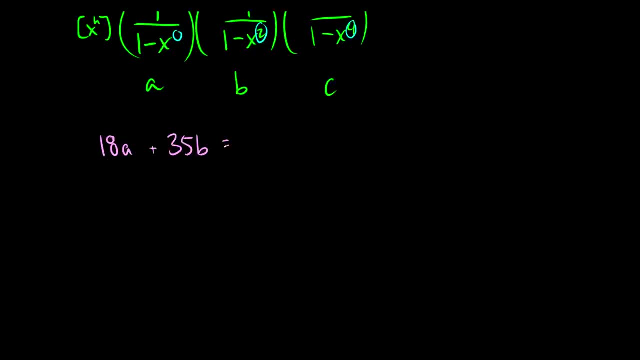 Plus 35b, equal to 96.. Okay, this is the same thing as saying I want the 96th coefficient of 1 over 1 minus x to the 18. Times 1 over 1 minus x to the 35.. 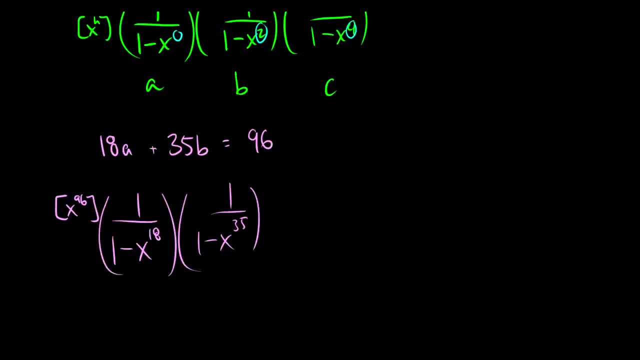 So when you understand the process of how we get to the generating function, it's very simple to take a look at one of these problems and say, okay, I know the generator, I know the generating function for this, But we can also throw some curveballs at you. 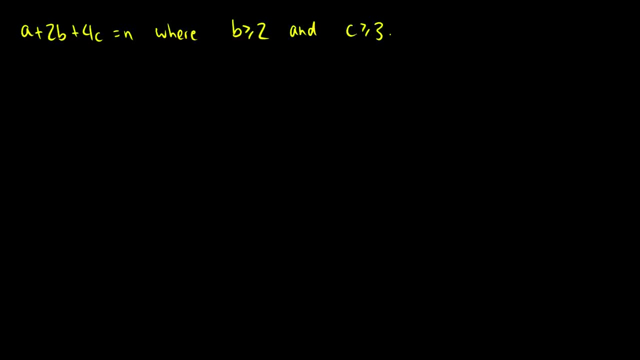 So here b has to be greater than or equal to 2.. And c has to be greater than or equal to 3.. Of course, this also implies that a is greater or equal to 0. So let's do a. a is going to be the same as before, because it's the same restrictions. 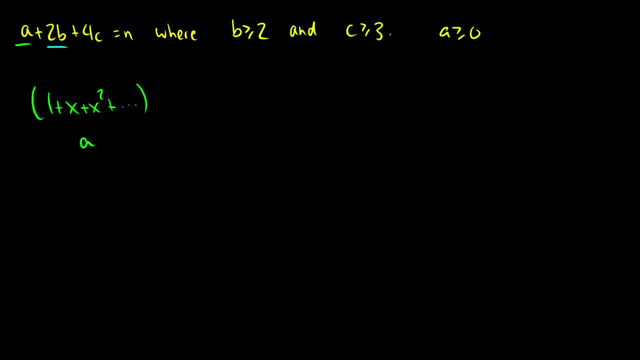 So that's our a, And our b is going to be 1 plus x squared Plus x4 plus x6 plus dot dot dot, just like before, But we have the restriction that b has to be greater than or equal to 2.. 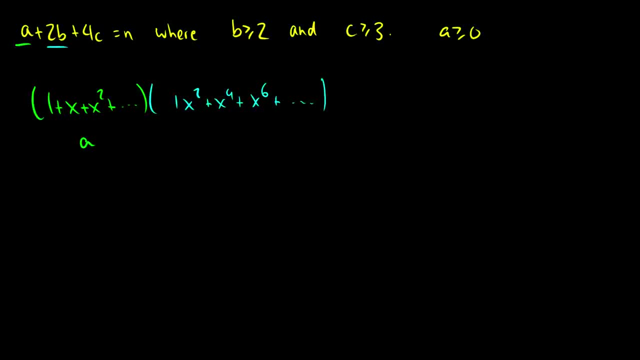 So we can't have the situations where we pick x to the 0.. And we can't have the situation where we have x squared. So what we do is we start at x4.. Why? Because we have to pick at least two objects. 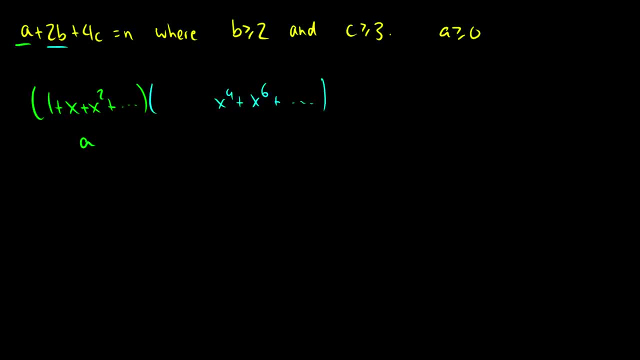 And 2 times 2 is 4.. So our smallest that we can pick here is x to the 4.. So what? we write this as x to the 4 plus x to the 8, plus dot, dot dot, And that's our b's. 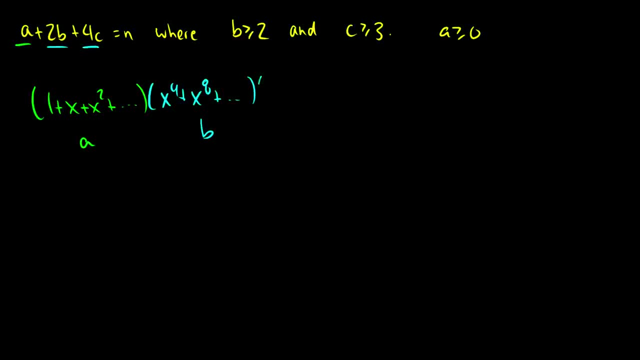 Our c's well, c has to be greater than or equal to 3.. So we can't pick one object, two objects or zero objects. We have to pick at least three objects. So what is 3 times 4?? 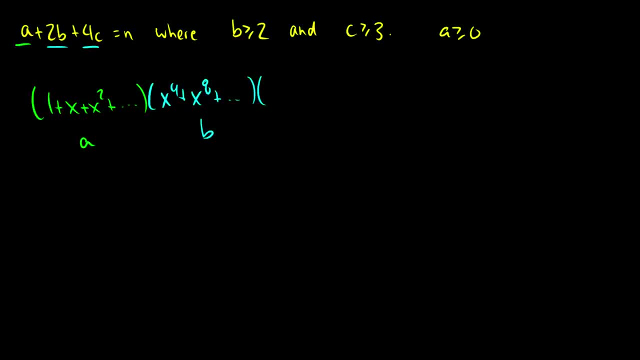 Because we have to pick at least 3.. And whatever we pick is multiplied by 4.. So the smallest, The smallest we can pick is x to the 12.. And this should be in pink. So the smallest we can pick there is x to the 12.. 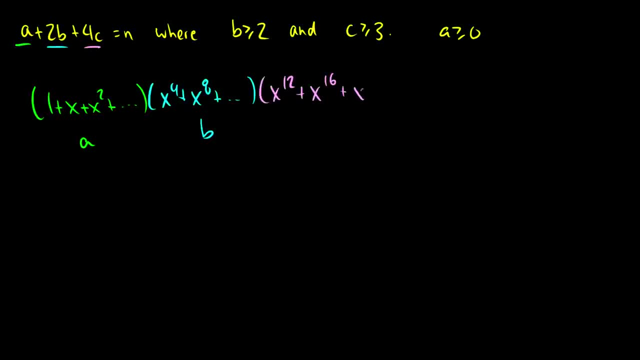 And then again it just goes up by 4s, because we're dealing with 4 times the constant. So that's our c's. Now we can simplify this. So our a is 1 over 1 minus x, Our b: we can factor out x to the 4.. 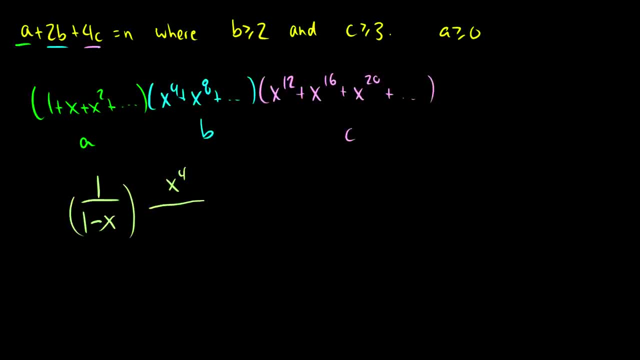 So we can shift it down to 1 plus x4 plus x8, so on, And that'll be over 1 minus x to the 4.. And sorry, you know what This b should be: x to the 6.. 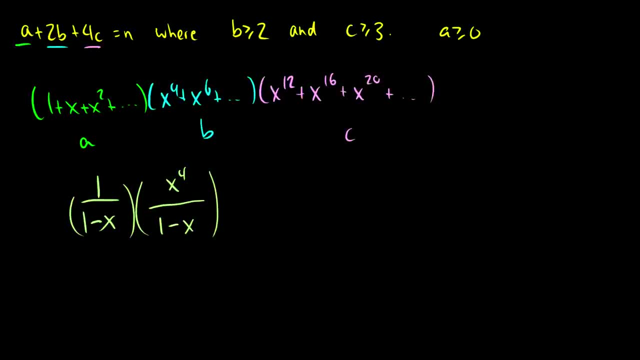 Because we're going up by 2s here. So we can shift that to x4 over 1 minus x squared And then our c's we can factor out an x12. And we can get 1 minus x to the 4 on the denominator. 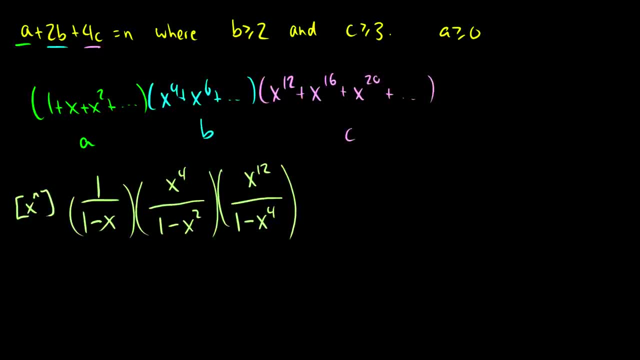 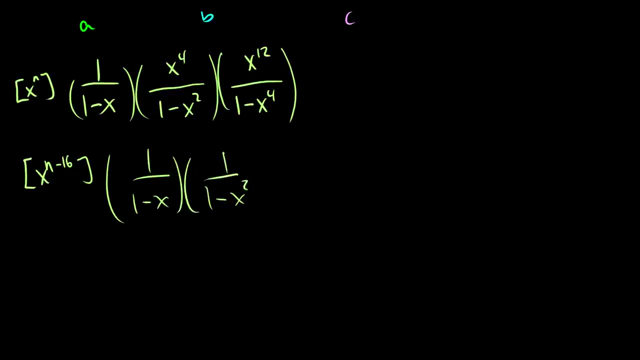 And what we want is we want, We want x to the n or the nth coefficient, So well, we can group up our x to the 4 and x to the 12. And we can do some shifting. So again we remember this is x to the n minus 16 of 1 over 1 minus x times 1 over 1 minus x, squared times 1 over 1 minus x to the 4.. 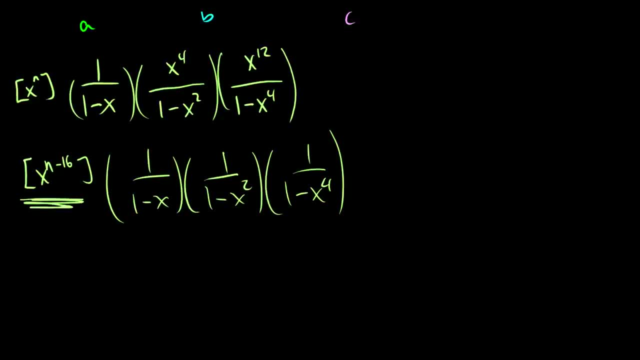 And if you don't know why this happened, well, we just grouped up x to the 4,, x to the 12.. And because when we multiply by a certain power of x, we just shift the generating function over, We're just shifting it back. 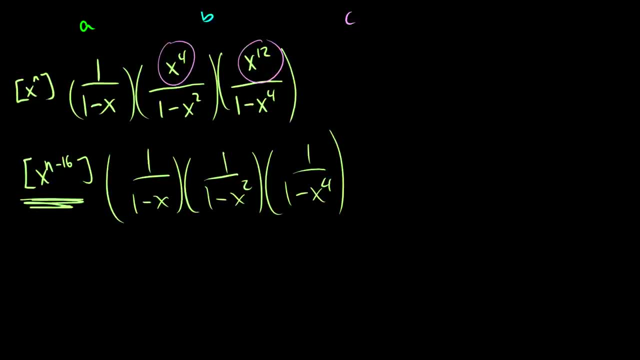 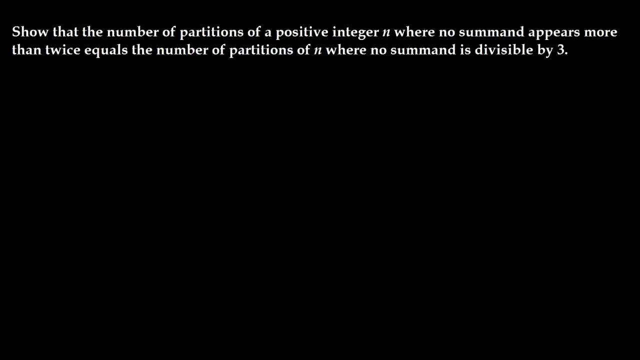 So that was explained in the previous video. There is one more thing we can do, And this was a problem in one of the textbooks that I use for this. So I figured: hey, this is somewhat difficult, Let's do it, Because I don't want a 10 minute video on something that is actually fairly challenging. 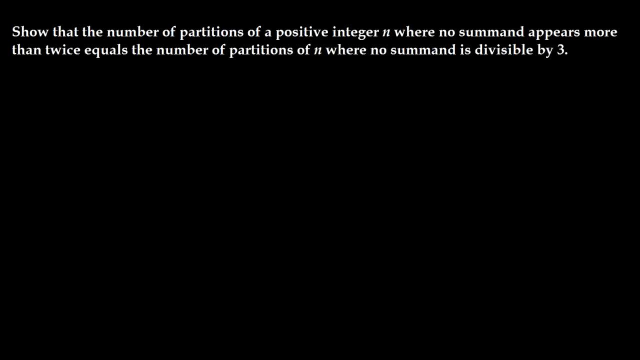 For For exams. And this is one of the questions. you see and you think I understand integer partitions, but I have no idea where to start here. So I want to show that the number of partitions of a positive integer where no summoned appears more than twice is equal to the number of partitions where no summoned is divisible by 3.. 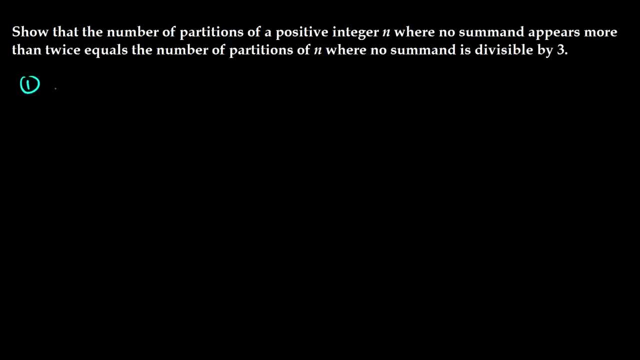 So first, this is none appear more than twice. So what that means is: we can only have 0,, 1, or 2 1s. We can only have 0,, 1, or 2, 2s. 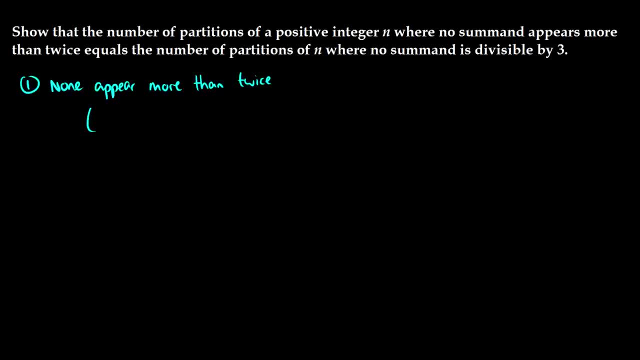 0,, 1, or 2, 3s. So for the 1s we get 1 plus x plus x squared, And that's the 1s. The 2s, we can get 0, 2s, 1, 2, or 2 2s. 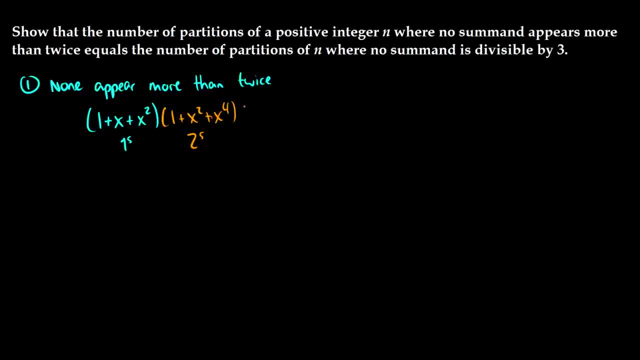 So those are the 2s, The 3s, The 3s are going to be 1 plus x, cubed plus x to the 6, because we can get 0,, 1, or 2 3s, and this will continue. 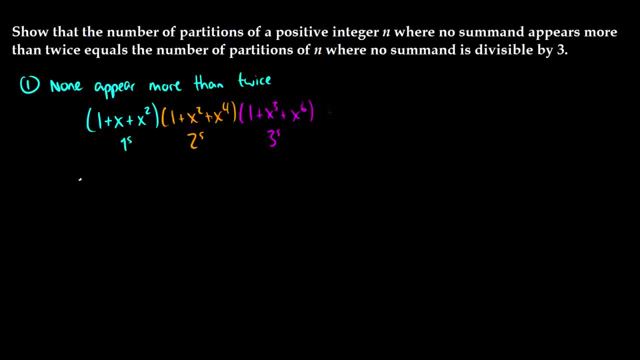 We can rewrite this as 1 minus x cubed over 1 minus x. if you remember the rules for generating functions, multiplied by 1 minus x to the 6 over 1 minus x squared, Our 3s can be 1 minus x to the 9 over 1 minus x cubed, and this will keep going. 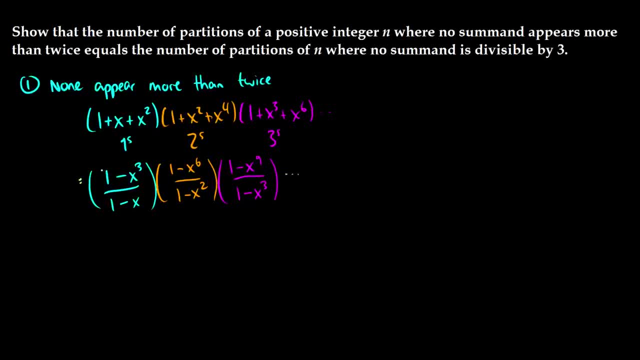 I did this just long enough to show you that this 1 minus x to the 3 will cancel with this denominator, And this chain is going to continue down over and over and over again. So what we get is going to be- I'll write it right here: 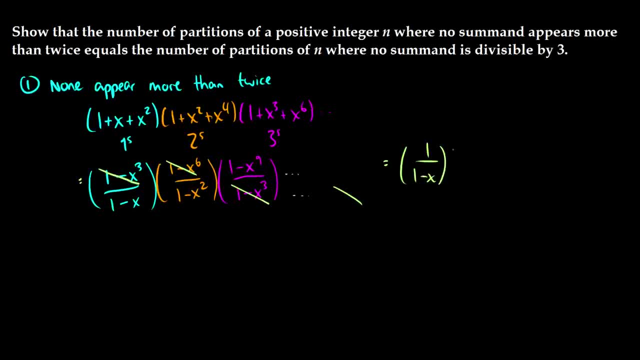 It's going to be 1 over 1 minus x times 1 over 1 minus x squared. The 1 minus x cubed over 1 minus x cubed will cancel out. So the next thing we get will be 1 minus x to the 4 times 1 minus x to the 5.. 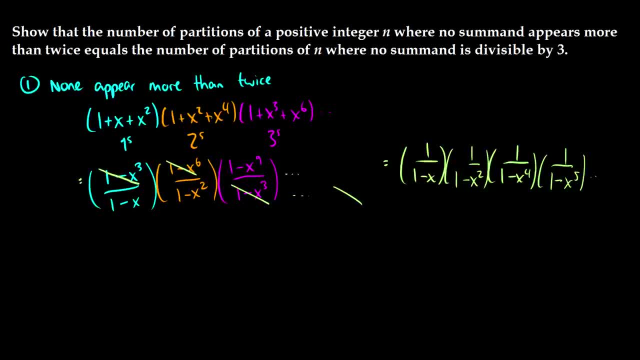 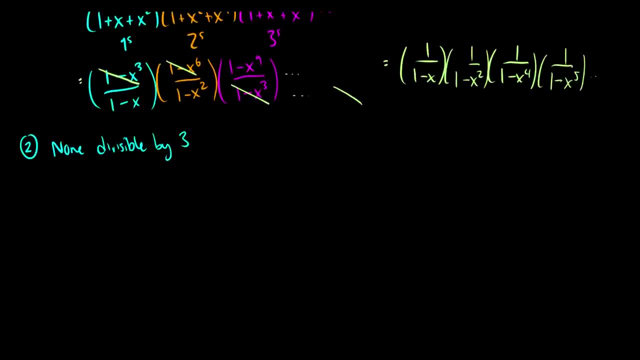 And that just keeps going. Now for the second part. we want none divisible by 3.. So what do we do here? Well, we want to show the scenario where none are divisible by 3.. So that means that we pick 1s. 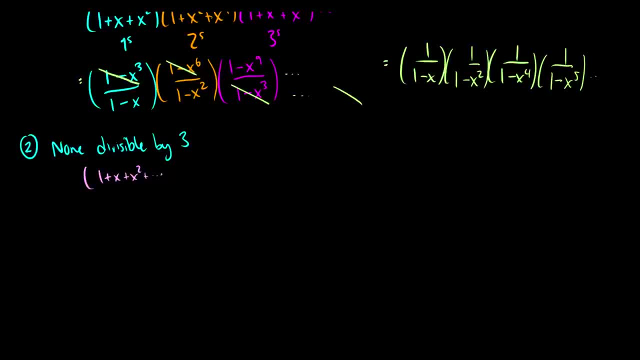 So we have 1 plus x plus x squared. We know our 1s, We know our 2s. So our 1 plus x squared, plus x to the 4, plus x to the 6.. So those are the number of 2s. 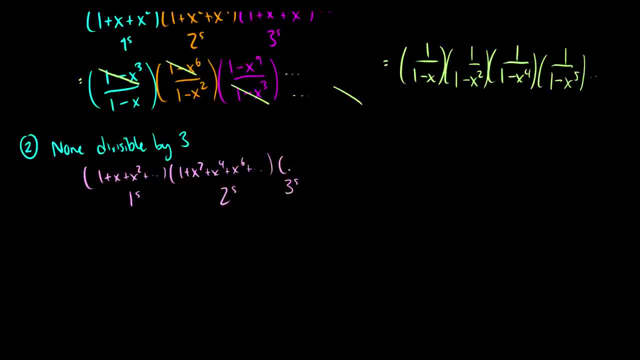 But for 3s we don't want to pick any, Because 3 is divisible by 3. So we just don't pick 1.. And then for the 4s we have 1 plus x to the 4, plus x to the 8, so on. 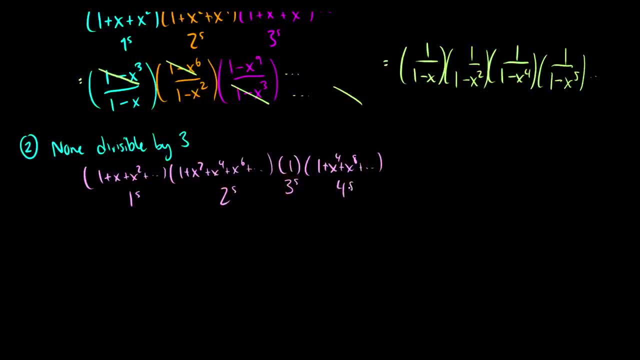 So we know, that's the 4s. The 5s are the same way. So let's just figure out the generating function for that. Well, the 1s is just 1 over 1 minus x. The 2s is 1 over 1 minus x, squared. 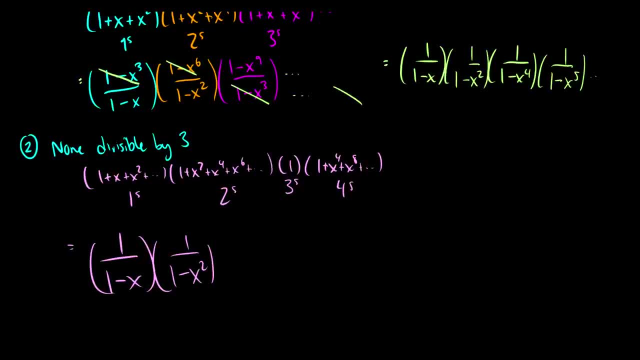 The 3s. well, we don't have 3s so we don't include it. The 4s is 1 over 1 minus x to the 4.. If we did a 5, it'd be 1 over 1 minus x to the 5.. 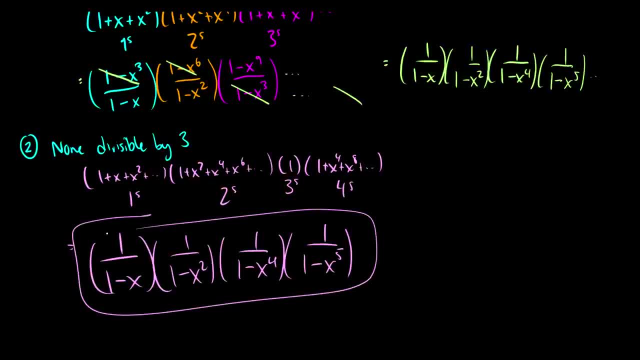 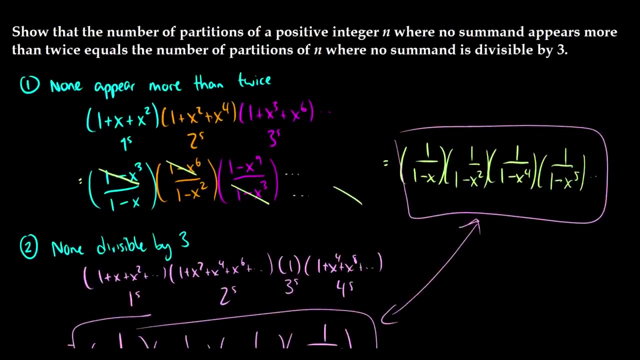 And you can see here that these two are exactly the same. So that's something we can show with generating functions. Show that the number of partitions of a positive integer n, where no sum appears more than twice, is equal to the number of partitions. 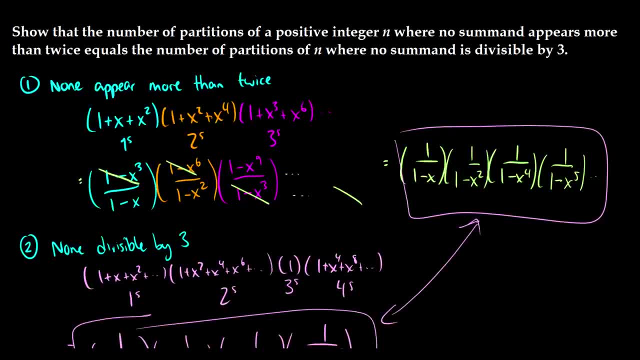 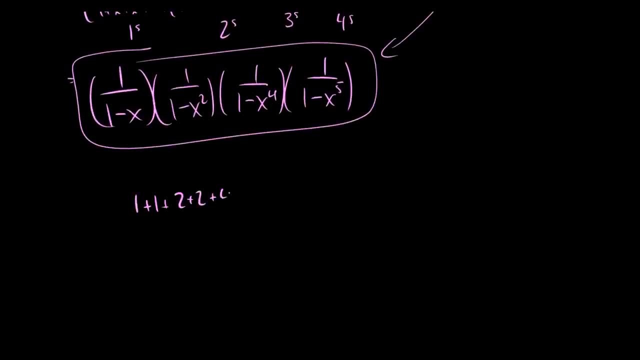 where no sum is divisible by 3.. So if we take a look, let's say we have 1 plus 1 plus 2 plus 2 plus 4 is equal to what's that? 10. The number of ways to get to 10, with all these summons appearing at most twice. 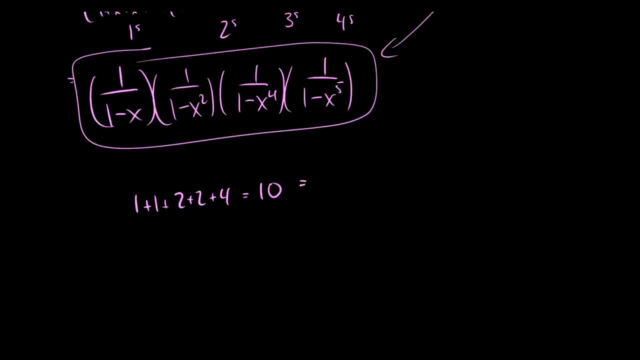 is the same way as the number of ways where none of them are divisible by 3.. So 5 plus 5 could be one of those Kind of cool. So that was integer partitions. Compositions are different. I won't be covering those yet, but I will cover compositions. 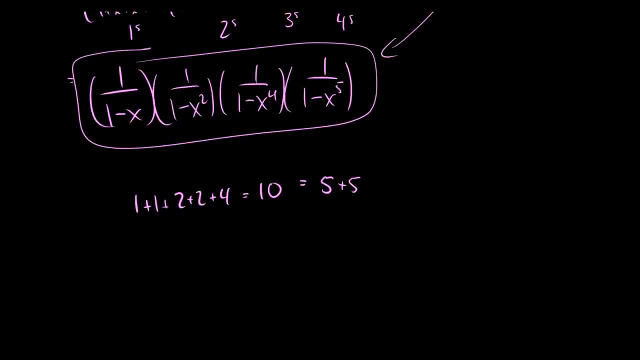 So that'll be later. If you have any questions, you can leave them in the comments here. You can go to trevtutorcom check out some of the other videos, or you can go to the subreddit at redditcom- slash r, slash- trevtutor and discuss questions there. If this helps you out, feel free.